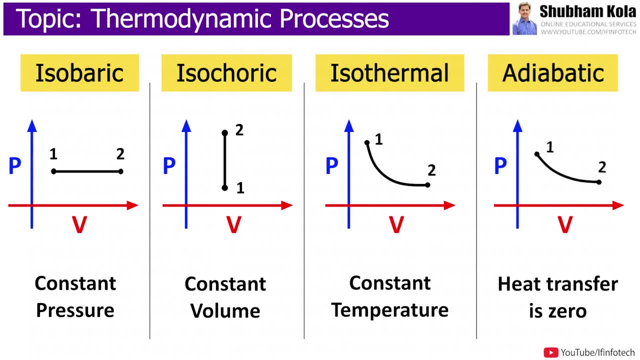 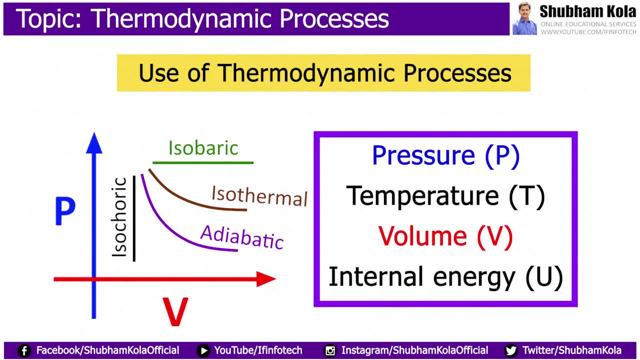 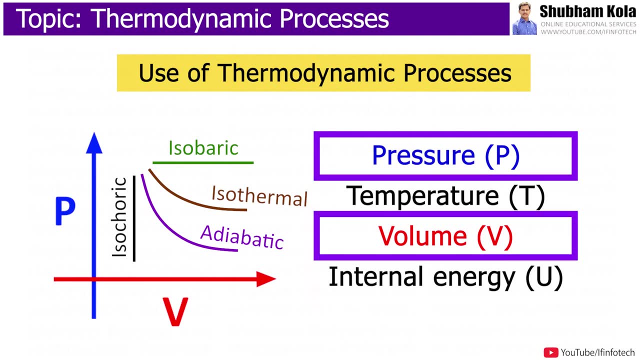 process where heat transfer is zero. So first we will understand what is the use of thermodynamic processes Here. the state of system can be expressed by various parameters, such as pressure, temperature, volume and internal energy. If any two parameters are fixed, like pressure and volume, or fixed mass of gas, the temperature. 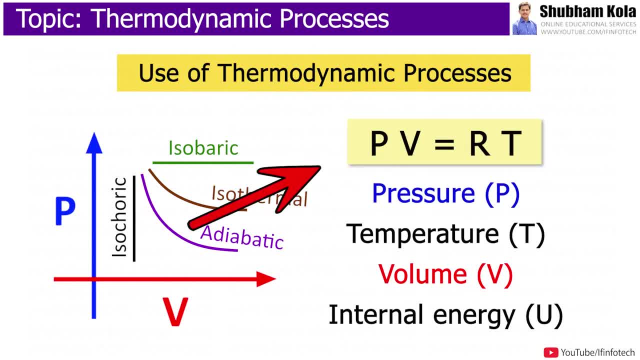 of gas will automatically fix. according to equation, PV is equal to RT. No change can be made to temperature without altering pressure and volume. By changing any of these parameters, the state of system can be changed. So the state of system can be changed by different thermodynamic processes. 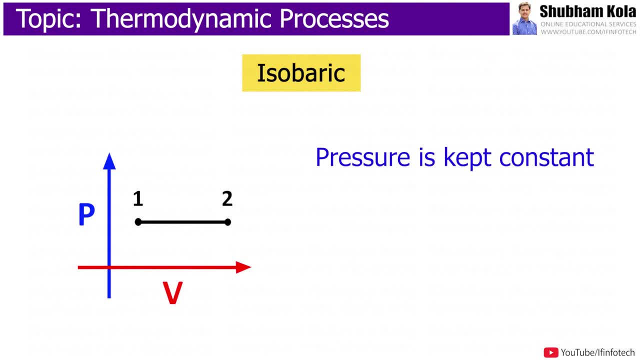 So here first is isobaric process, in which pressure is kept constant. Since the pressure is constant in this process, the volume of system changes And work done can be calculated by the equation: W is equal to P multiplied by change in volume, that is, V final minus V initial. 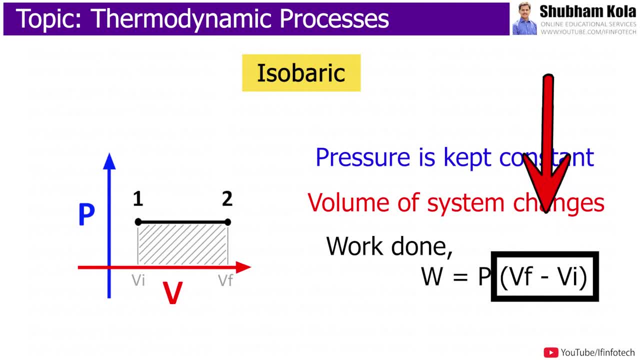 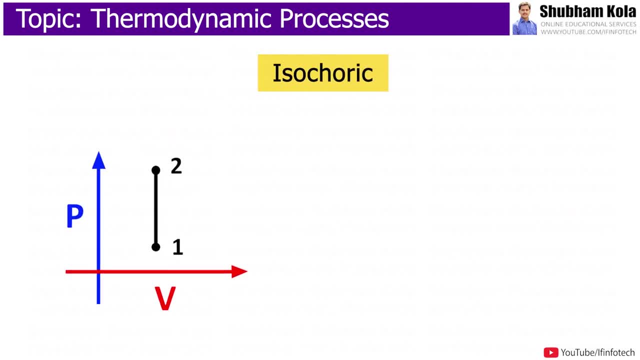 If change in volume is positive, that is expansion, the work done is positive. and for negative change in volume, that is contraction, the work done is negative. In isochloric process, the volume remains constant. Therefore, system does not do any work. 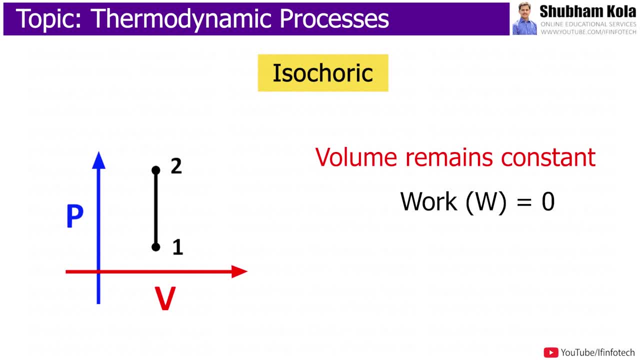 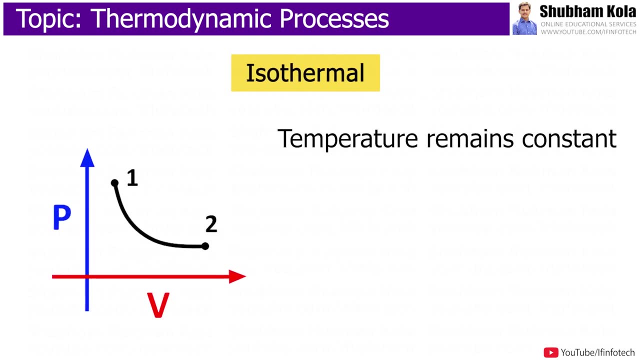 Such process, in which there is no change in volume, can be achieved by placing thermodynamic system in closed container which neither contracts nor expands. Thus, from the first law of thermodynamics, change in internal energy becomes equal to heat transfer. Now, in isothermal process, the temperature of system remains constant. 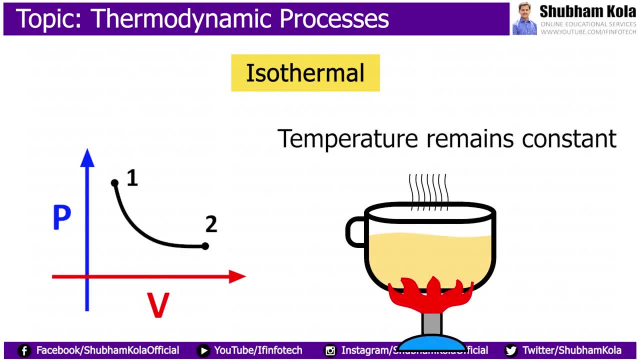 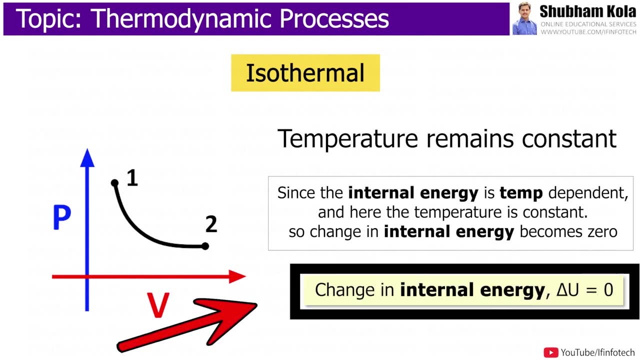 This process occurs when system is in contact with outside thermal reservoir and change in system will occur slowly to allow the system to continue to adjust to temperature of reservoir through heat exchange. And since the internal energy is temperature dependent and here the temperature is constant, so change in internal energy becomes zero. 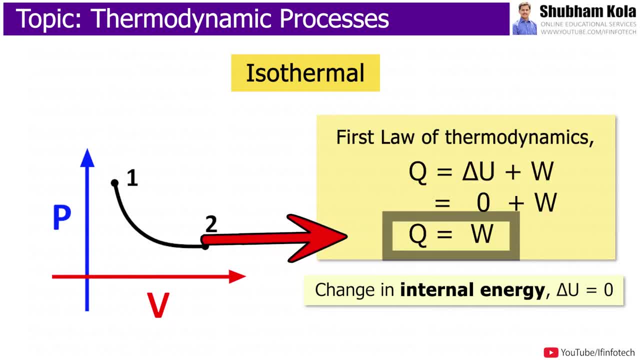 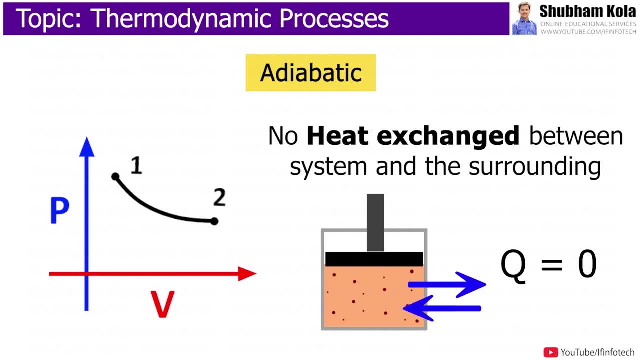 And thus from the first law of thermodynamics we will get: Q is equal to W. In adiabatic process no heat exchange between system and surrounding, so Q is equal to zero. So adiabatic process occurs without transmitting heat and mass between system and surrounding. 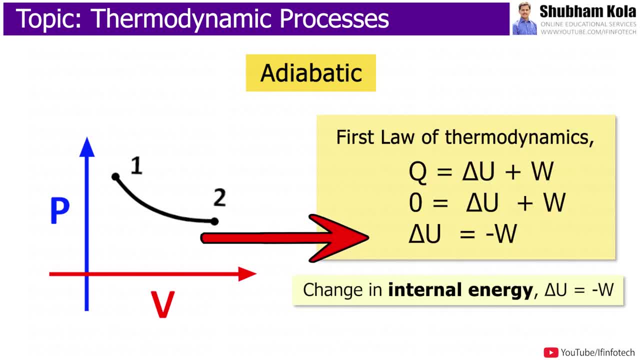 Since Q is equal to zero for an adiabatic process, from the first law of thermodynamics we will get: change in internal energy is equal to negative work done. Thus, internal energy will increase if the work done is negative, and vice versa.